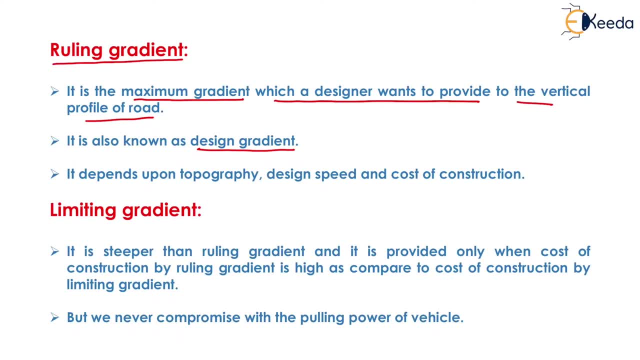 It is also known as design gradient. It depends upon topography, design, speed and cost of construction. Now the second gradient is falling gradient. The next gradient is the limiting gradient. It is steeper than rolling gradient and is provided only when cost of construction by rolling gradient is high as compared to the cost of construction by limiting gradient. 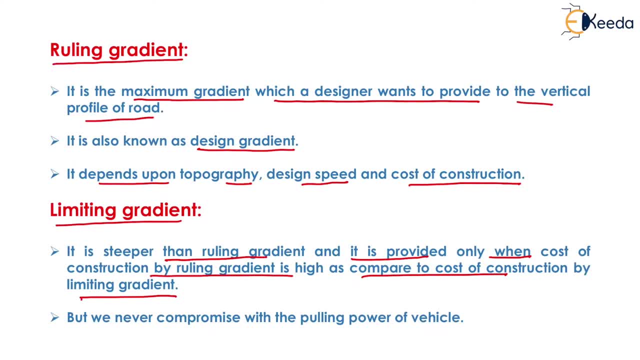 It means that we will provide limiting gradient in case when the cost of construction by rolling gradient is very high. So we will provide limiting gradient there, But we never compromise with the pulling power of the vehicle. It means that the gradient will. 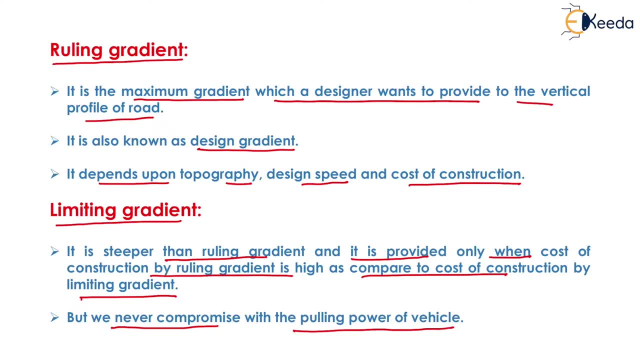 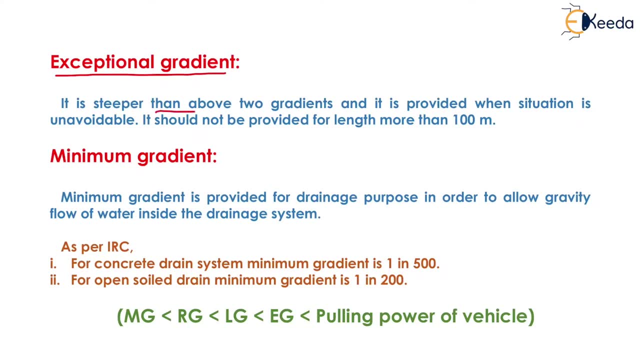 always be less than the pulling power of the vehicle. Otherwise vehicle will not travel along that gradient. Now the next is the exceptional gradient. It is steeper than above two gradients and it is provided when situation is unavoidable. It should not be provided for length more than 100 meter. 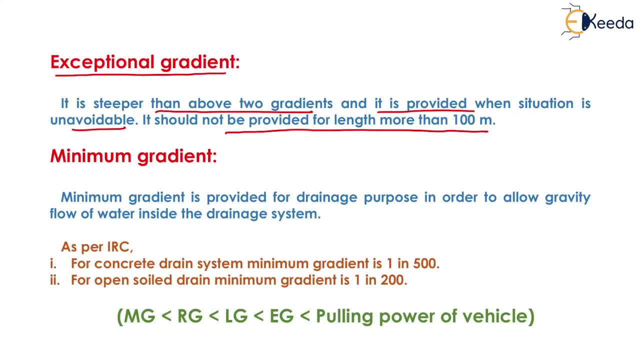 It means that when the situation is unavoidable and we have to connect the two vertical points by a steeper gradient, then we have to provide the exceptional gradient, And it should not be provided for length more than 100 meter. Now, the next is the minimum gradient. 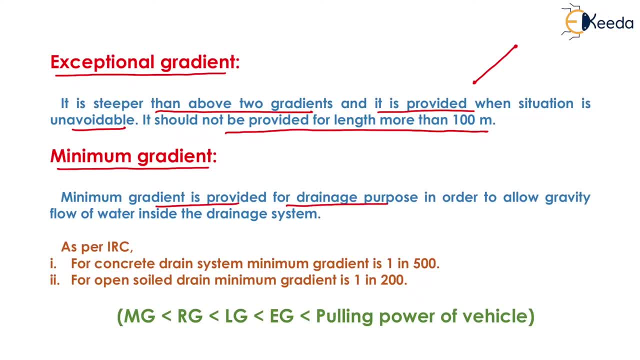 Minimum gradient is provided for drainage purpose in order to allow gravity flow of water inside the drainage system. It means that the minimum gradient is only provided for the drainage purpose. As per Indian Road Congress for concrete drainage system, minimum gradient is 1 in 500.. 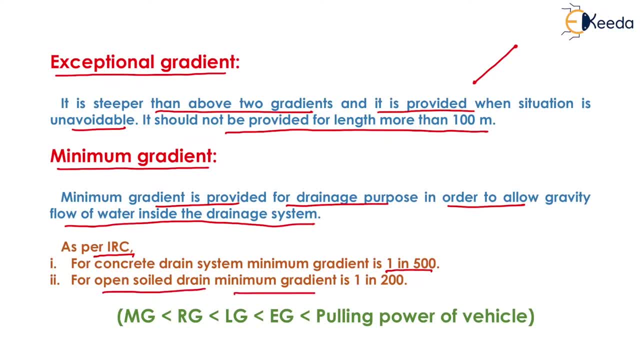 As per Indian Road Congress, for concrete drainage system, minimum gradient is 1 in 500.. And for open soil drain, minimum gradient is 1 in 200.. Minimum gradient will be less than rolling gradient And rolling gradient will be less than limiting gradient. 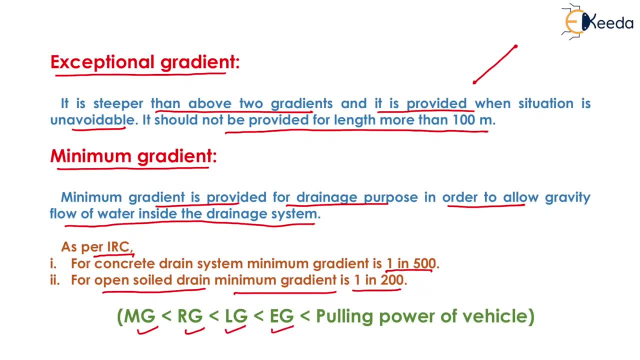 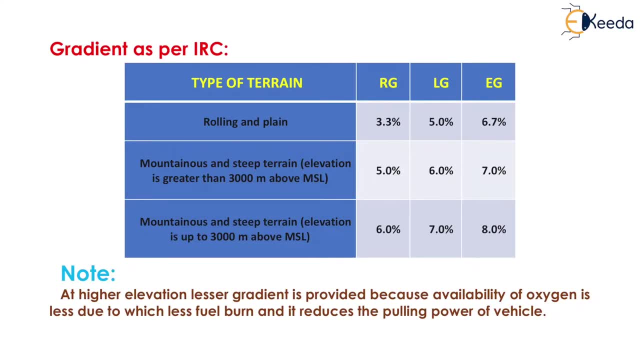 And limiting gradient will be less than exceptional gradient And all the gradients will be less than pulling power of the vehicle. Now in this table we had written the gradient as per the Indian Road Congress for different types of terrain. For rolling and plain terrain, rolling gradient is 3.3%. 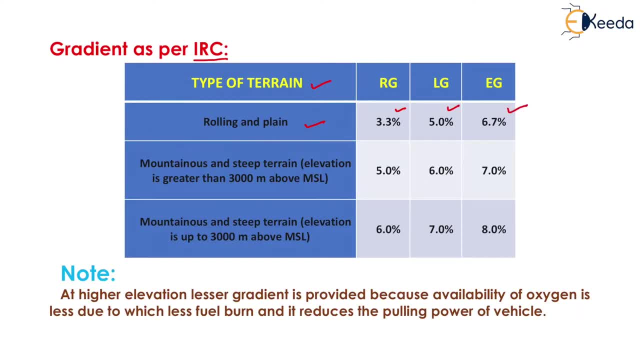 Limiting gradient is 5% And exceptional gradient is 6.7%. Similarly, for mountainous and steep terrain, when elevation is greater than 3000 meter above mean sea level, then rolling gradient will be 5%, limiting gradient 6% and exceptional gradient 7%. 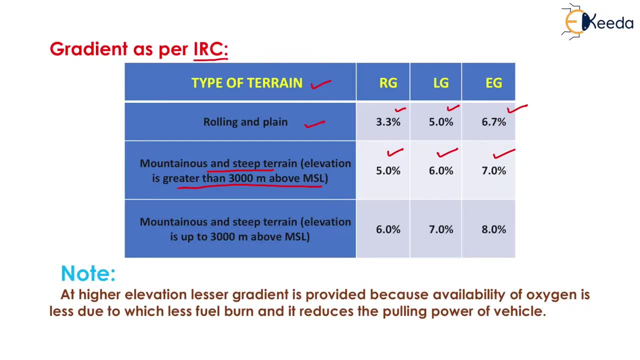 And for mountainous and steep terrain case, when the elevation is up to 3000 meter above MSL, then rolling gradient will be 6%, limiting gradient 6%. Limiting gradient will be 7% And exceptional gradient will be 8%. 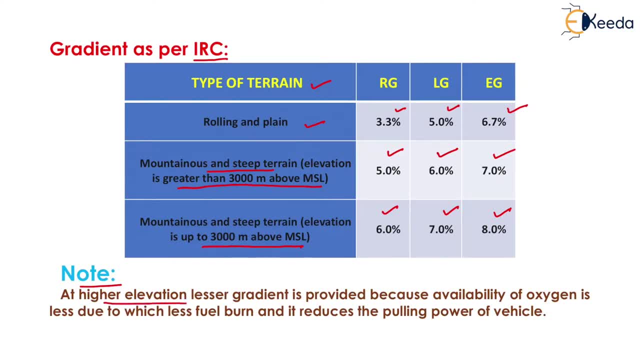 Now one note is written here: that at higher elevation lesser gradient is provided, which is shown here. That is, at higher elevation lesser gradient is provided Because availability of oxygen is less, due to which less fuel burn and it reduces the pulling power of vehicle. 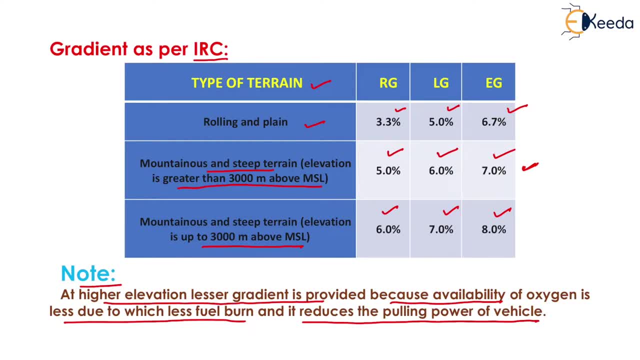 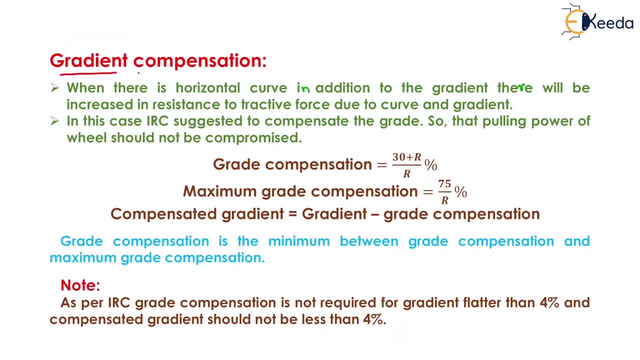 So if the availability of oxygen is very less at very high altitude, then it reduces the pulling power of the vehicle. So to counteract this effect we have to reduce the gradient at higher elevation Now. the next will be the gradient compensation. 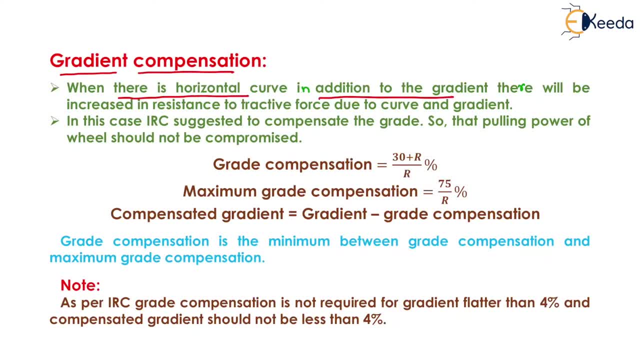 When there is horizontal curve in addition to the gradient, there will be increased in resistance to tractive force due to curve and gradient. It means that when there is a horizontal curve in addition to the gradient then it will reduce the pulling power. 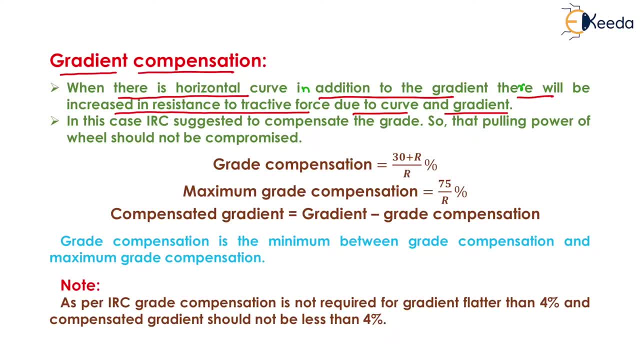 So it will reduce the pulling power of the vehicle because it will provide resistance to the tractive forces. In this case, IRC suggested to compensate the grade so that pulling power of vehicle should not be compromised. Now grade compensation will be equals to 30 plus r upon r, where r is the radius of the curve. 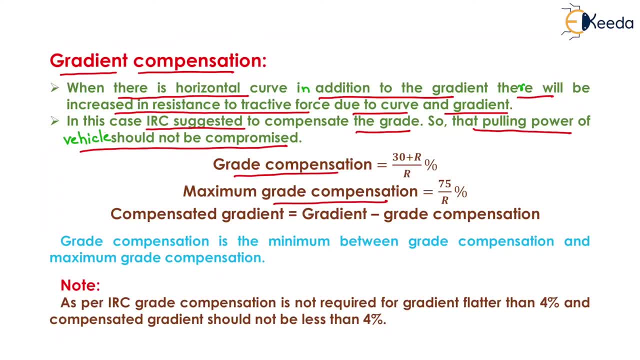 Maximum grade compensation will be equals to 75 upon r. Now we have to select one value which is the minimum of both these values. Now, we have to select one value which is the minimum of both these values. Now, compensated gradient will be equals to the gradient which is already given in the question, minus grade compensation. 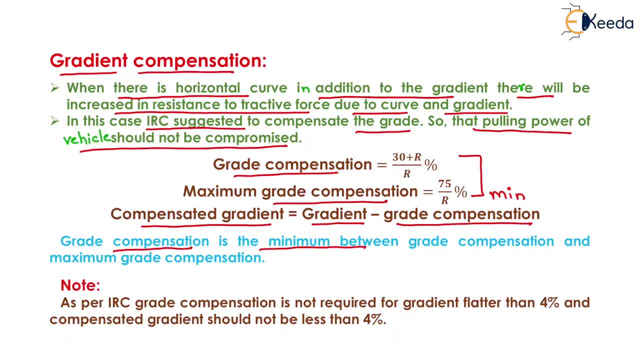 So grade compensation is the minimum between the grade compensation and maximum grade compensation which we had seen here. Now one note is there that, as per Indian Road Congress, grade compensation is not required for gradient flatter than 4%. It means that when the gradient is flatter than 4%, 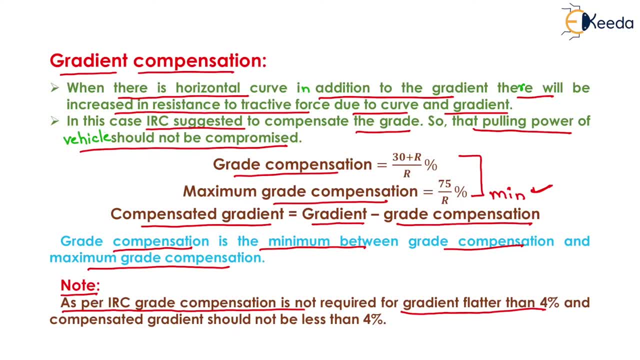 it means that when the gradient is flatter than 4%, then we don't require any grade compensation, And compensated gradient should not be less than 4%. It means that the minimum value of compensated gradient will be equals to 4%. 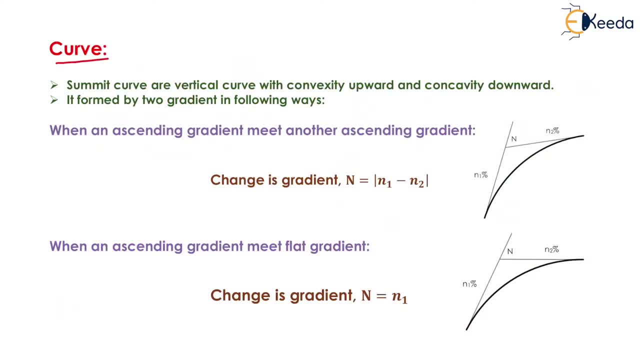 Now next vertical alignment is the curve. Summit curves are vertical curves with convexity upward and concavity downward, like this: It is formed by two gradients in following ways: The first one will be when an ascending gradient meets another ascending gradient, like this: 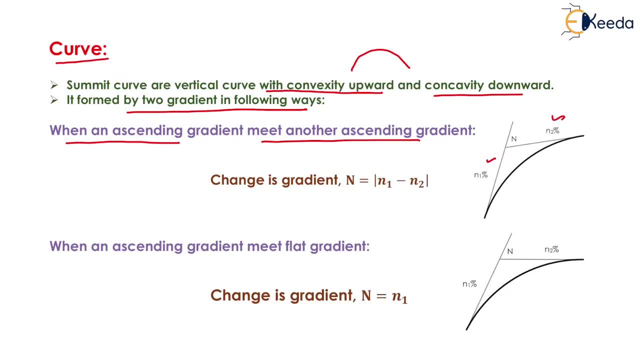 That is plus n1% and plus n2%. So change in gradient that is n, will be equals to modulus n1 minus n2, which is written here Now. the second case will be when an ascending gradient meets flat gradient. 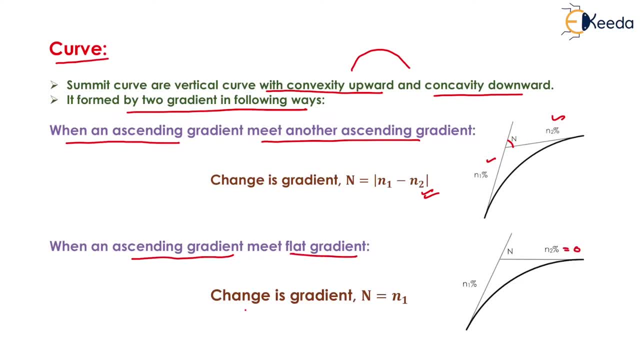 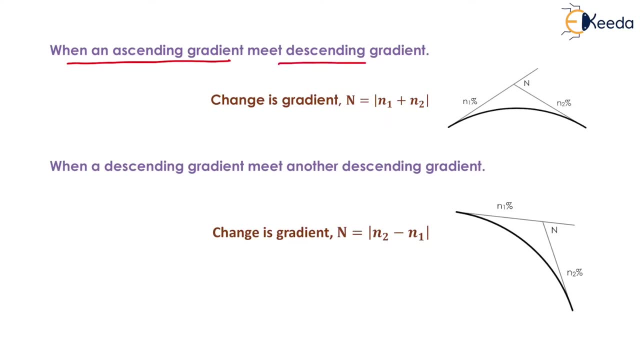 it means that the value of n2 will be equals to 0. So change in gradient will be equals to n1 only Now. the third case will be when an ascending gradient meets descending gradient, which is shown here. That is, plus n1% and minus n2%. 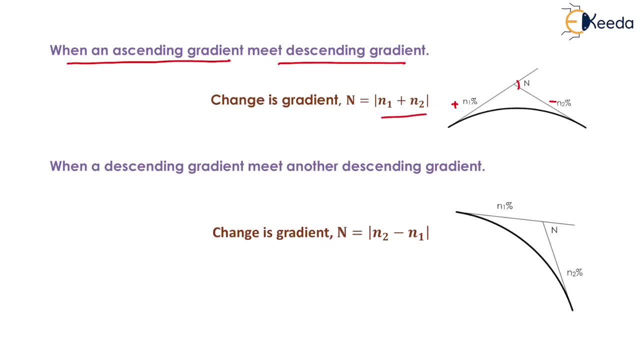 So n will be equals to n1 plus n2.. When a descending gradient meets another descending gradient, that is the case 4.. So here minus n1% and minus n2% will be the gradient. So change in gradient capital N will be equals to in modulus n2 minus n1.. 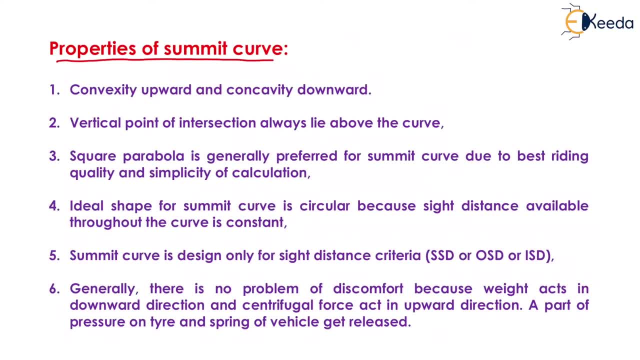 The properties of summit curve. Generally, summit curve have convexity upward and concavity downward, like this: That is the summit curve. Vertical point of intersection always lies above the curve. It means that the vertical point of intersection will always lies above the curve, like this: 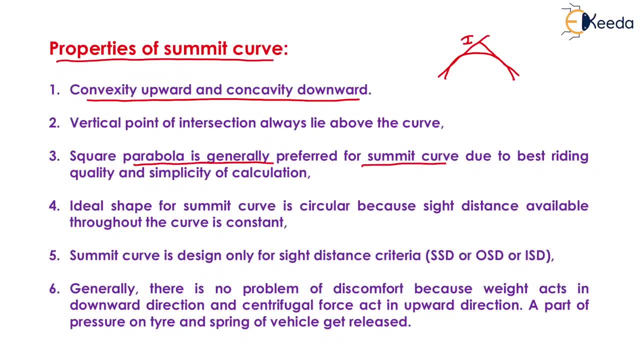 Square parabola is generally preferred for summit curve due to the best riding quality and simplicity of calculation. It means that for summit curve the best profile is the square parabola. Ideal shape for summit curve is circular, because side distance available throughout the curve is constant. 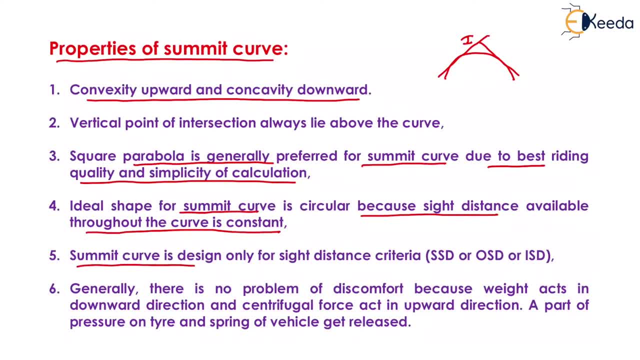 Now the next property is summit curve is designed only for side distance criteria, That is, for SSD, that is, stopping side distance or overtaking side distance or intermediate side distance. Generally there is no problem of discomfort because weight acts in the downward direction. 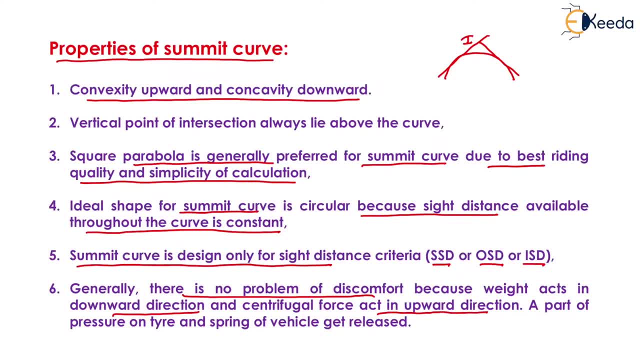 and centrifugal force acts in the upward direction. It means that when vehicle is travelling along this summit curve, then weight will be acting in this direction, that is, W, and centrifugal force will be acting in this direction, that is, in upward direction. 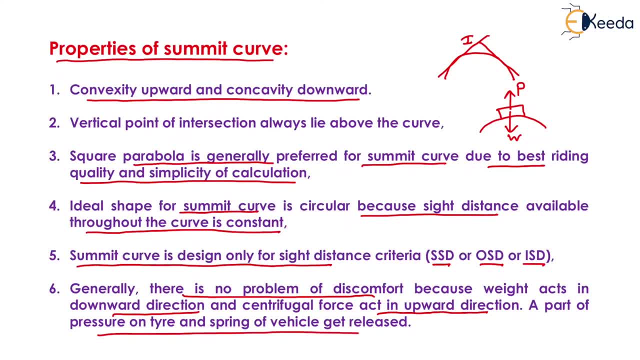 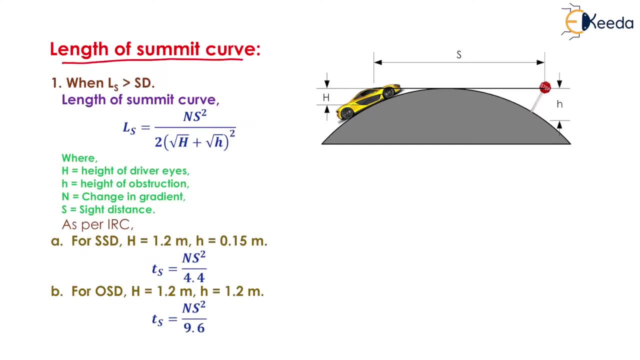 A part of pressure on tyre and spring of vehicle get released due to this type of force. Now we have to find the length of summit curve. The first case will be when length of summit curve is greater than side distance. It means that 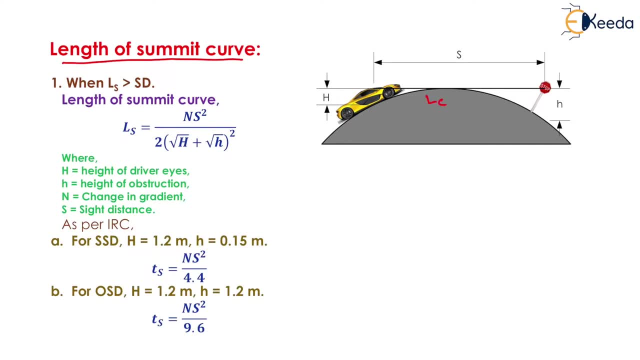 when the length of curve which is shown here is greater than the side distance, Then length of summit curve will be equals to ns square upon 2 in bracket, root capital H plus root small h, whole square Where capital H is the height of driver I. 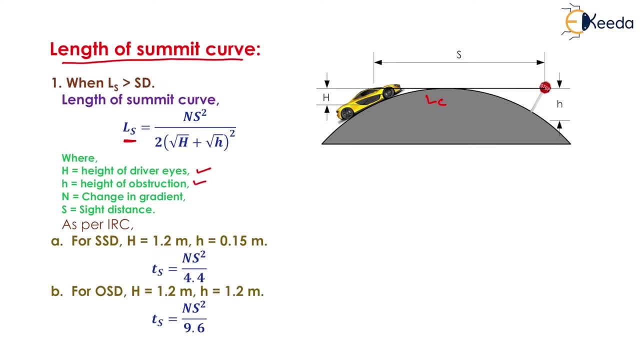 small. h will be the height of obstruction, Capital, N will be change in gradient and S is the side distance. Now, as per Indian Road Congress for stopping side distance, we know that height of driver I is 1.2 meter and height of obstruction is 0.15 meter. 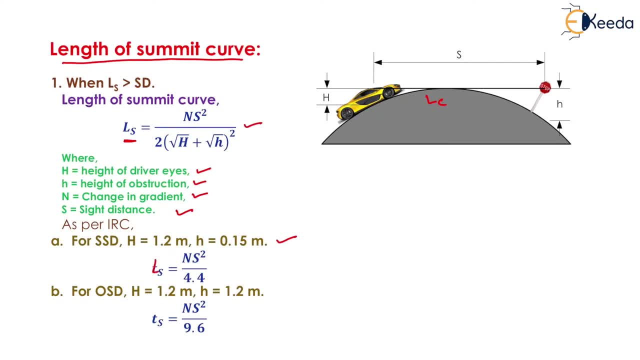 On putting this value in this equation, the length of summit curve will be equals to ns, square upon 4.4.. Similarly, for overtaking side distance, we know that height of driver I is 1.2 meter and height of obstruction is also 1.2 meter. 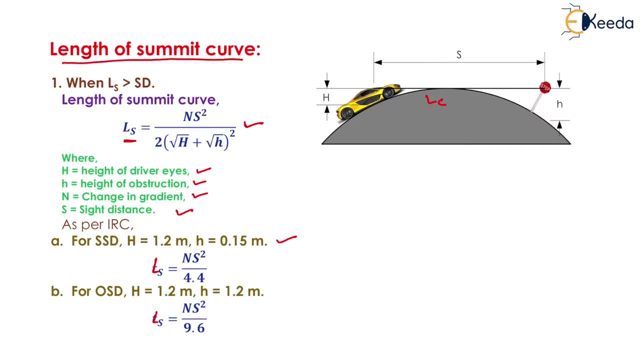 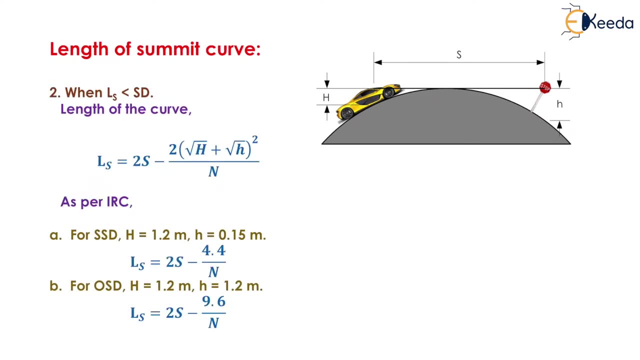 On putting this value in the above equation, the length of summit curve will be equals to ns, square upon 9.6.. Now case 2.. When length of summit curve is less than side distance, then length of summit curve will be equals to: 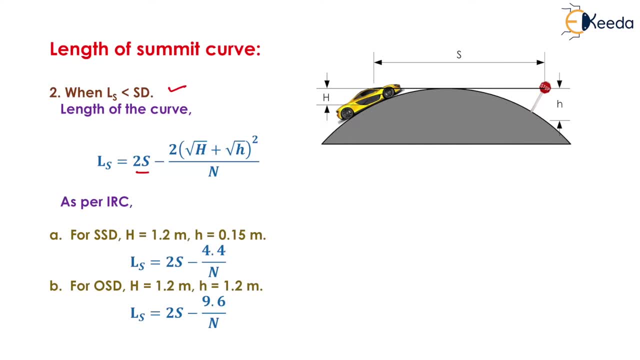 2s minus 2 in bracket. root capital H plus root, small h, whole square upon capital N. Now for stopping side distance. we will put capital H value as 1.2 meter and small h value equals to 0.15 meter. 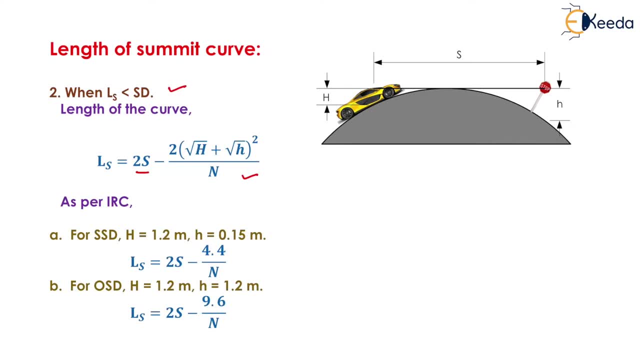 So we will get the length of summit curve as 2s minus 4.4 upon N. Similarly, for overtaking side distance, Ls will be equals to 2s minus 9.6 N. Now one note is there, that 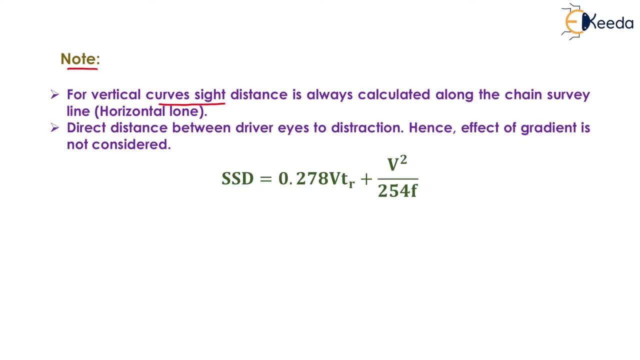 for vertical curves, side distance is always calculated along the chain survey line, That is the horizontal line. Direct distance between driver I is 2 destruction. Hence effect of gradient is not considered in the calculation of stopping side distance. So we had removed the gradient from the equation. 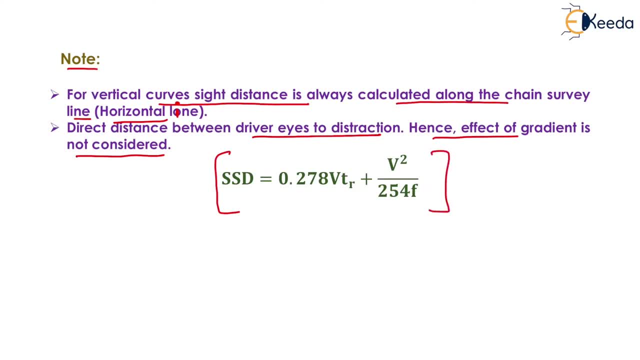 So the equation will be: Ls is equal to 2s minus 9.6 N From the equation. so the equation will become: 0.278 V into T R, where T R is the reaction time and V is the speed of the vehicle. 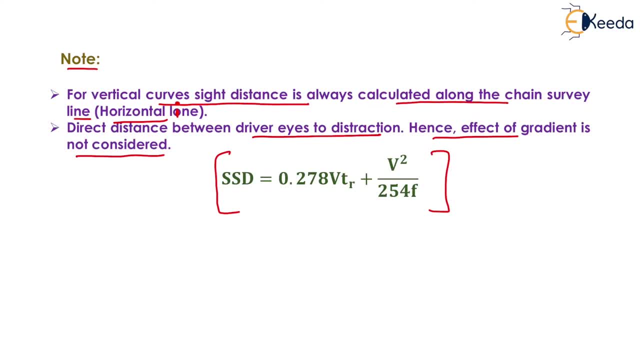 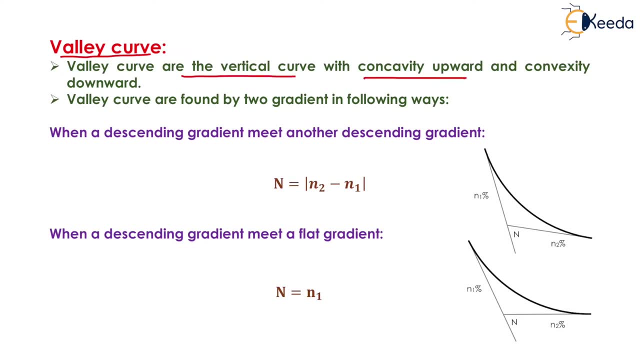 plus V square upon 254 F. F is the coefficient of friction. Now the next curve is the valley curve. Valley curves are the vertical curves with concavity upward and convexity downward, just like this. Valley curves are found by two gradients in following ways. 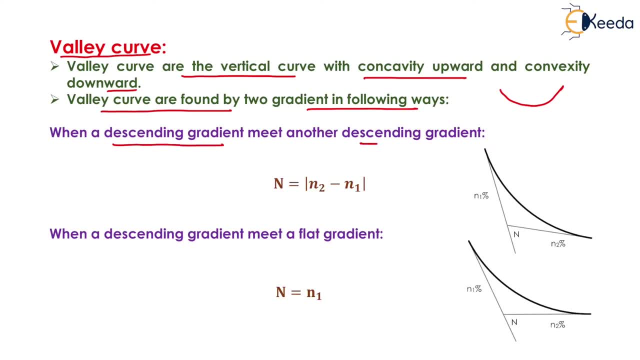 The first one will be when a descending gradient meets another descending gradient. it means that minus N1 percent and minus N2 percent, So N will be equal to N2 minus N1.. Similarly, when a descending gradient meets a flat gradient, 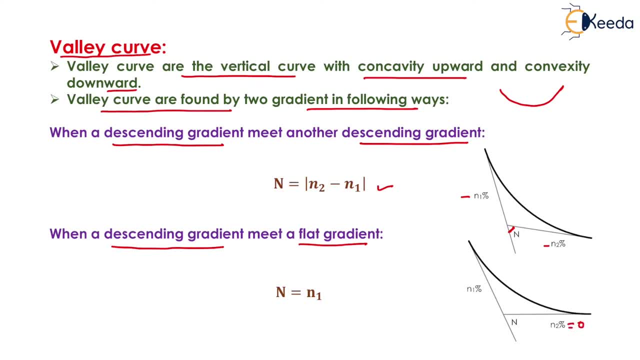 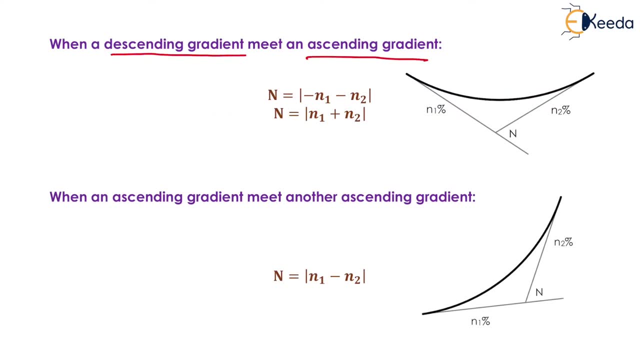 it means that the value of N2 will be equal to 0. So N will be equal to N1. only Third case will be when a descending gradient meets an ascending gradient. then N will be equal to N1 plus N2.. 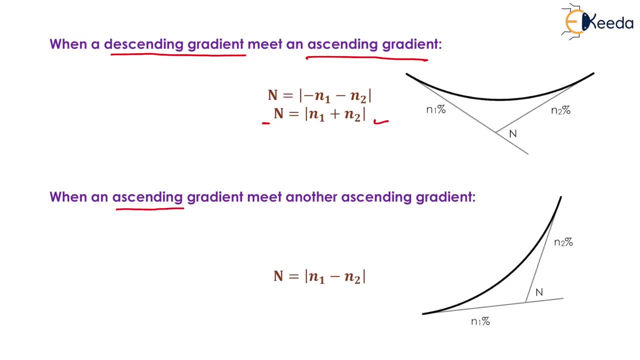 Similarly, the fourth case will be when an ascending gradient meets another ascending gradient. that is, plus N1 percent and plus N2 percent. So N will be equal to N1 minus N2.. Now properties of valley curve: Concavity upward and convexity downward. 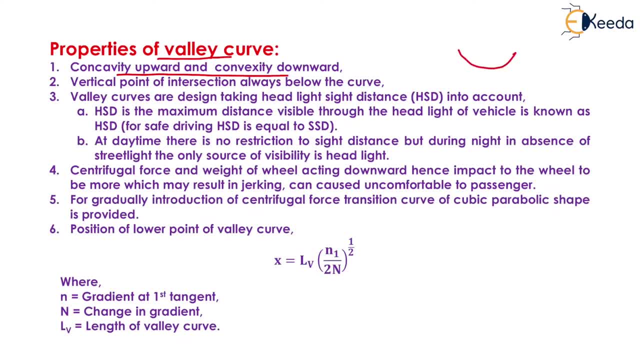 which we had already seen. like this, Vertical point of intersection always lies below the curve. It means that the vertical point of intersection always lies below the curve, which is shown here. Valley curves are designed taking headlight set distance into account. Headlight set distance is the maximum distance visible. 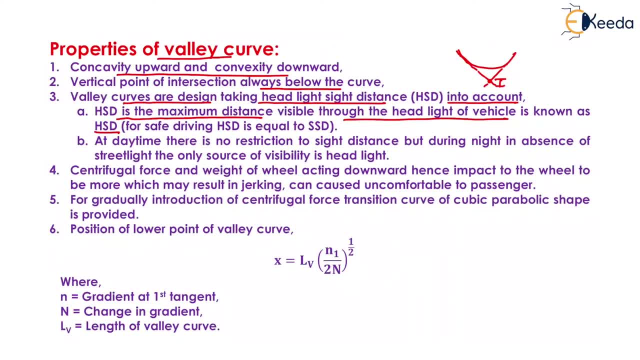 through the headlight of vehicle is known as headlight set distance. For safe driving, headlight set distance is always equal to the stopping set distance. At daytime, there is no restriction to set distance, but during night, in absence of street light, 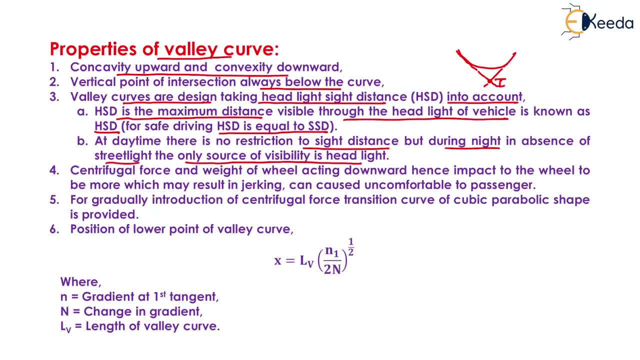 the only source of visibility is headlight, Centrifugal force and weight of wheel acting downward, hence impact to the wheel to be more, which may result in jerking. Now, when a vehicle is travelling along a valley curve like this, 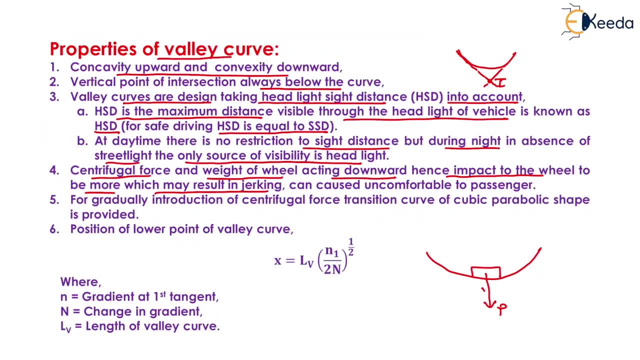 then centrifugal force and weight, both will be acting in the downward direction, due to which it can cause uncomfortability to the passengers. For gradual introduction of centrifugal force transition curve of cubic parabola shape is generally provided. Position of lower point of valley curve is given as: 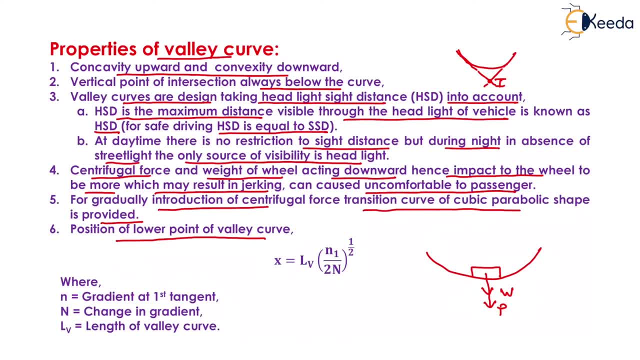 X equals to length of valley curve, that is, LV n1 upon 2 into capital N to the power 1 by 2, where n1 is the gradient of first tangent. capital N equals to change in gradient. LV equals to length of valley curve. 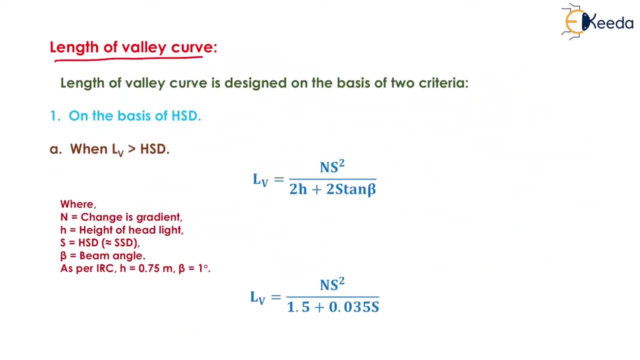 Length of valley curve can be determined by the following cases, that is, on the basis of headlight set distance. when length of valley curve is greater than headlight set distance, then length of valley curve will be equals to ns square upon 2h plus 2s tan beta. 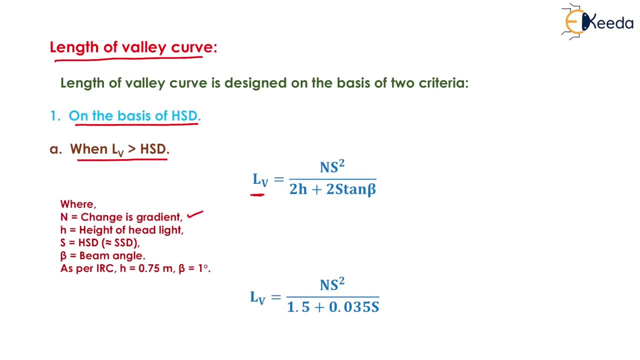 Here, capital N is the change in gradient, h is the height of headlight, s is the headlight set distance, which is generally taken to be equal to stopping set distance. beta is the beam angle s per Indian Road Congress, beam angle will be equals to 1 degree. 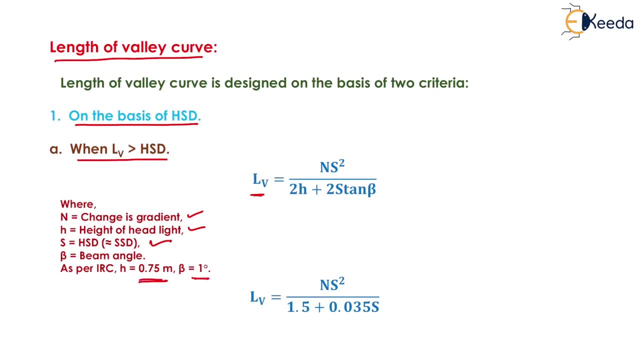 and h will be equals to 0.75 meter. On putting this value in the above equation, we will have length of valley curve equals to ns, square upon 1.5, plus 0.035s. Now, when length of valley curve is less than headlight set distance. 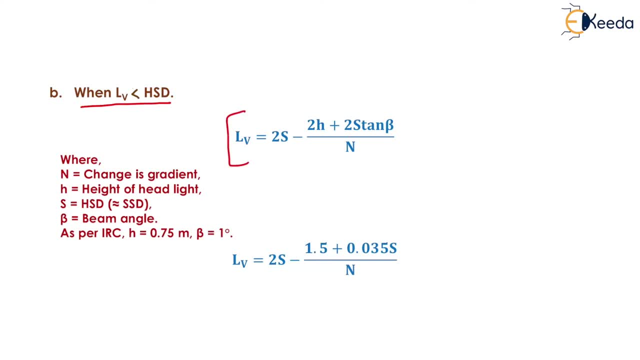 then length of valley curve will be equals to 2s minus 2h plus 2s tan beta upon n. On putting the value of h equals to 0.75 meter and beta equals to 1 degree, the length of valley curve will be equals to.